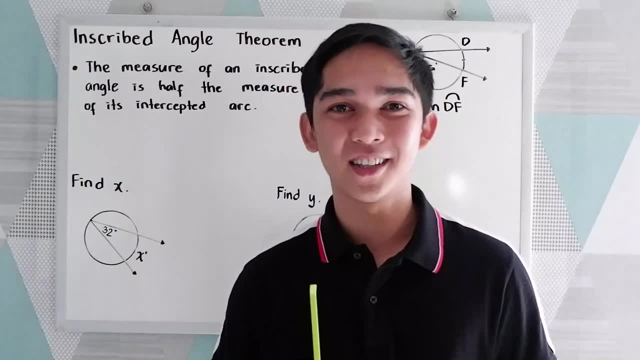 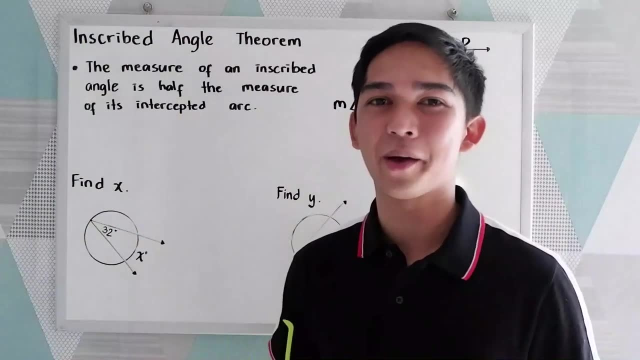 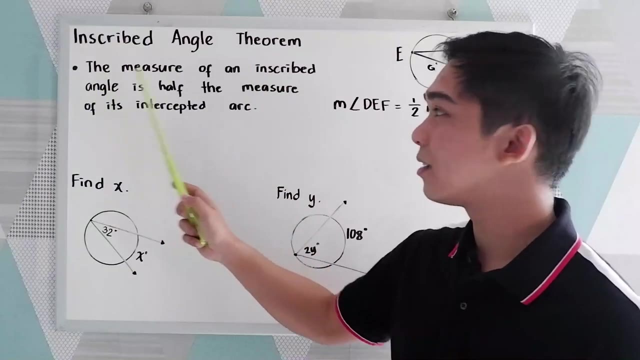 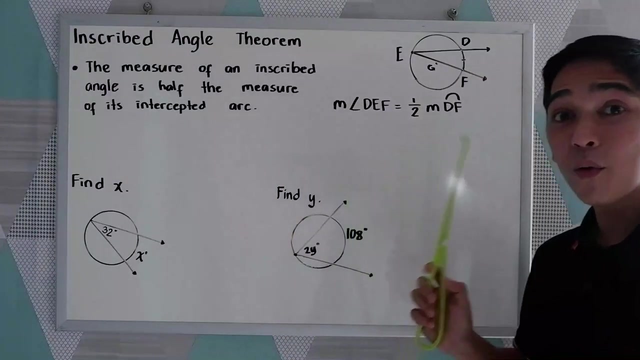 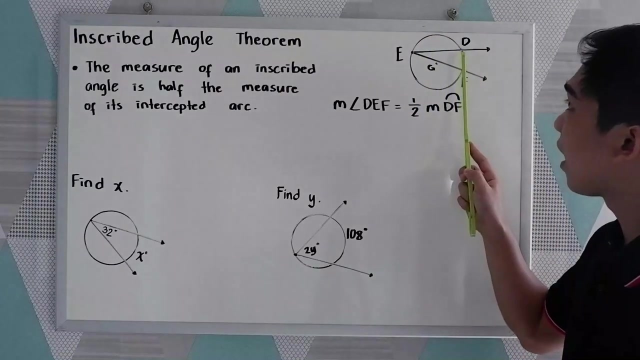 Good day everyone. welcome to Senior Pablo TV And for today's tutorial video. we will be discussing the Inscribed Angle Theorem. This theorem states that the measure of an inscribed angle is half the measure of its intercepted arc. We have our diagram here, the circle G, And we have an inscribed angle which is DEF and the intercepted arc. 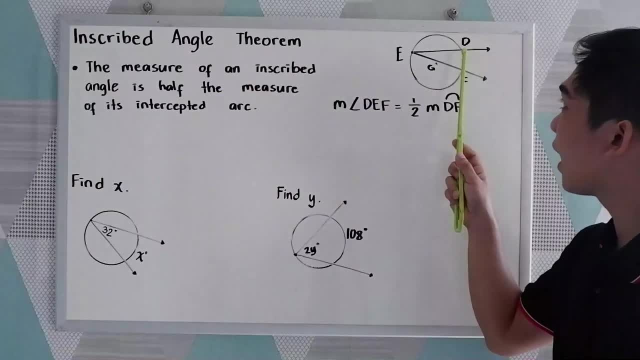 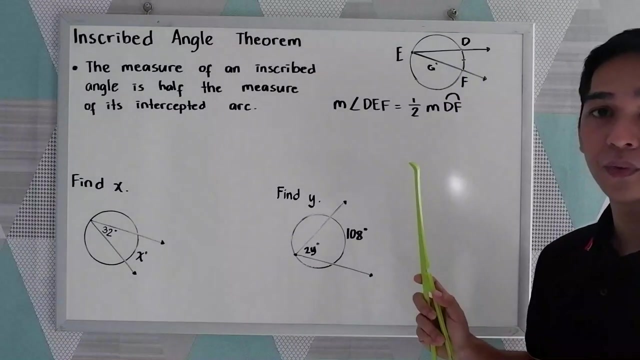 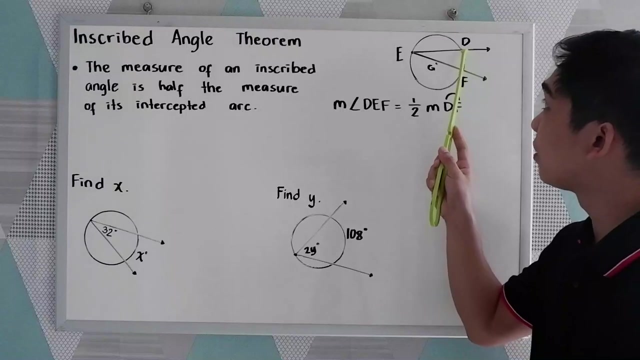 Following our theorem, to find the measure of the inscribed angle, DEF, that is equal to half of the measure of the intercepted arc, which is DEF. Let's say our DEF here is 60.. So this is 60.. This is 60.. 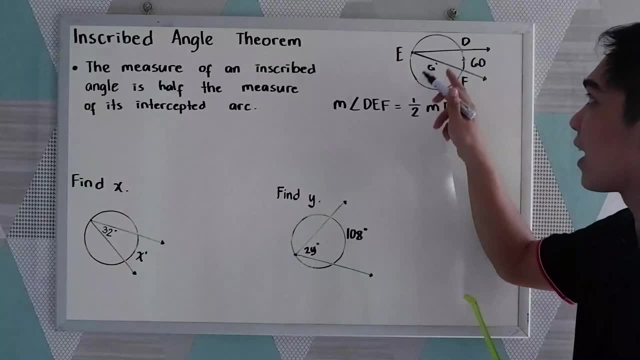 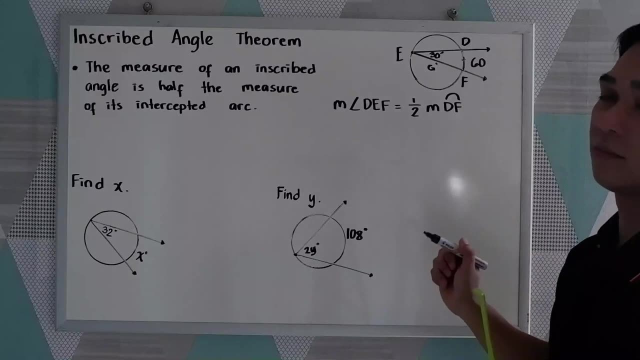 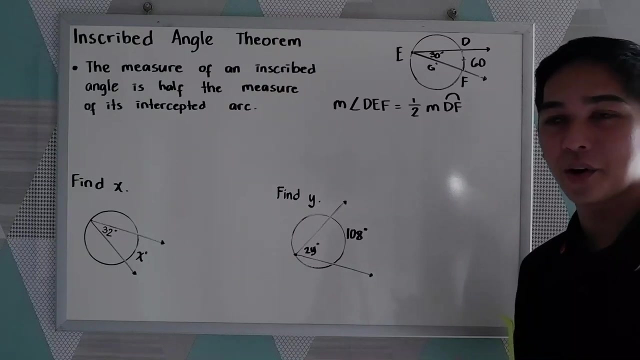 Therefore the measure of DEF angle DEF is half of this measure, So this will become 30.. So 60 divided by 2. That is 30.. So that is the Inscribed Angle Theorem. Let's have the following examples: 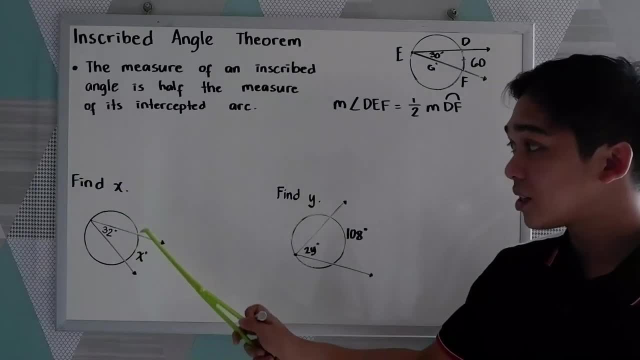 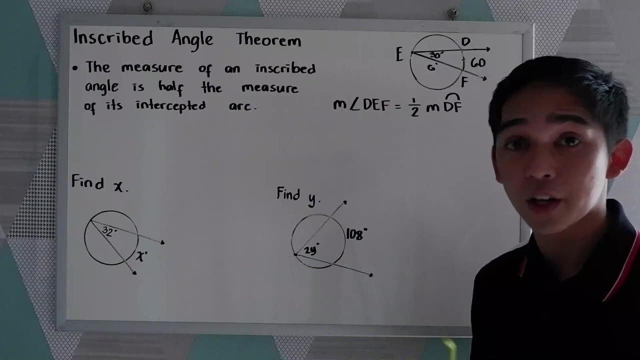 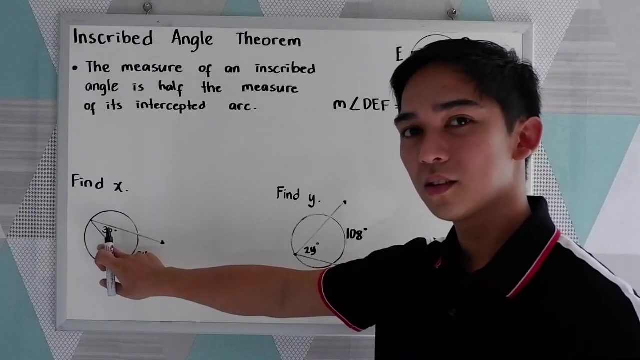 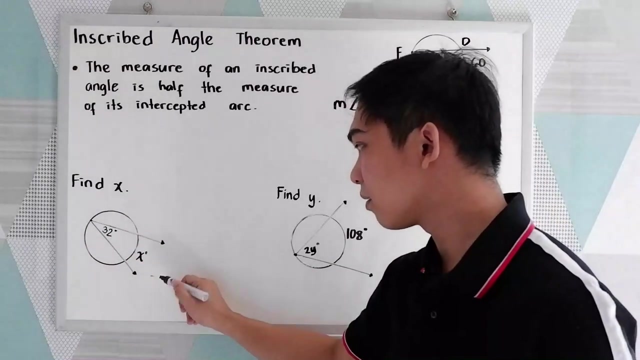 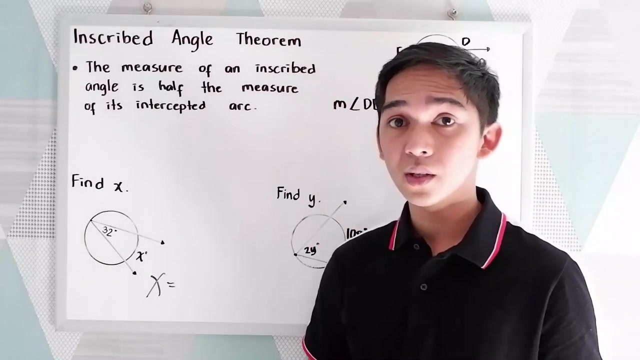 Our first example is Find X using this illustration, And the second one is Find Y using this second illustration. Let's find X, So 62, following our theorem, X, will be times 2.. So 32 times 2, that is 64.. 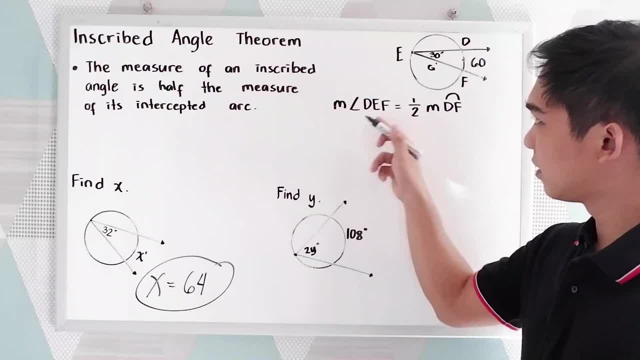 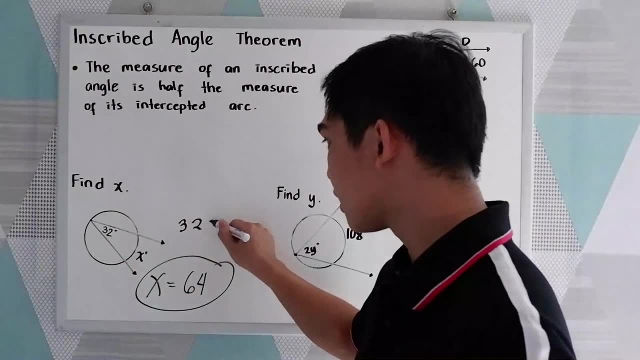 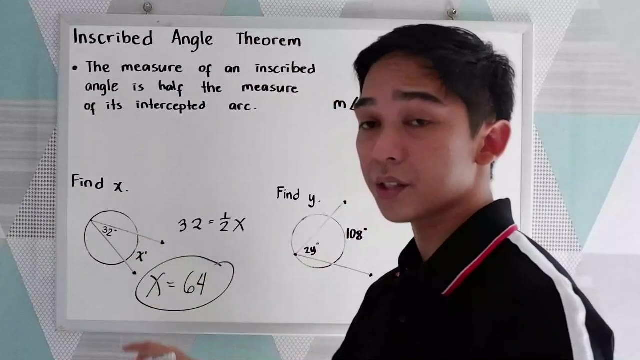 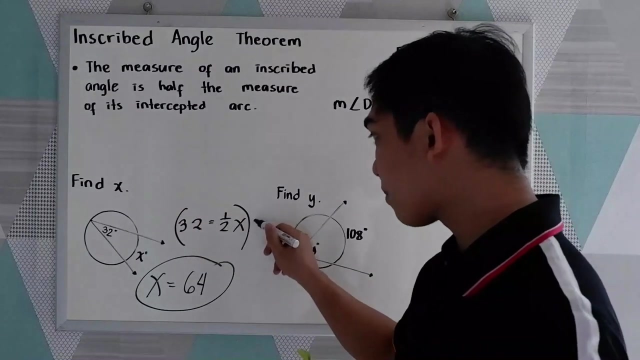 Next, So you can use the theorem. Okay, let us use the theorem. The measure of the angle, which is 32, is equal to one half of the intercepted arc. So our intercepted arc is 32.. A is X. Now to find X, we can multiply by 2.. 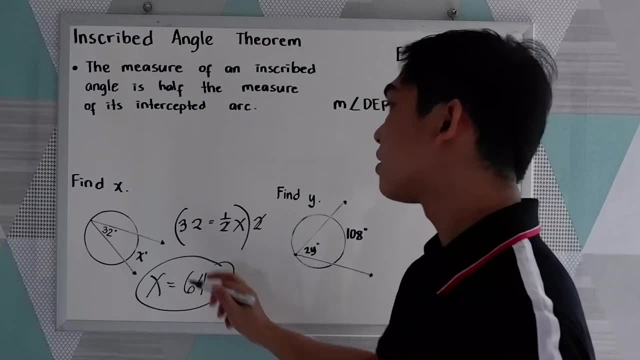 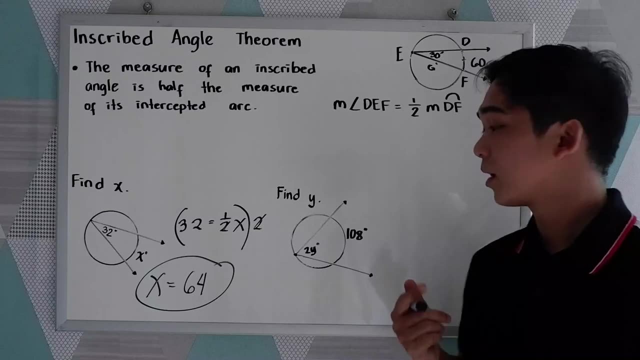 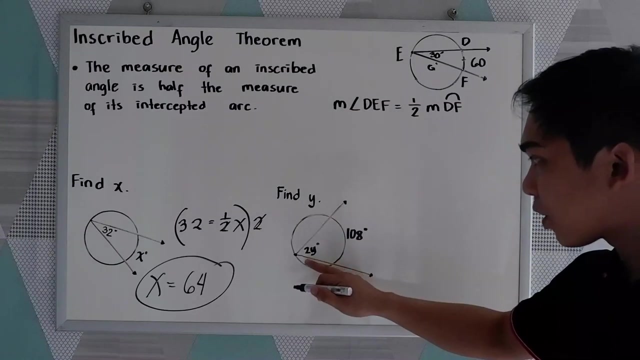 So this will be cancelled out. The theorem meaning is X Now 32 times 2,, which is 64. Or you can use mental calculation. In this case Find Y. We are looking for Y. So the measure of the angle is 2Y is equal to. 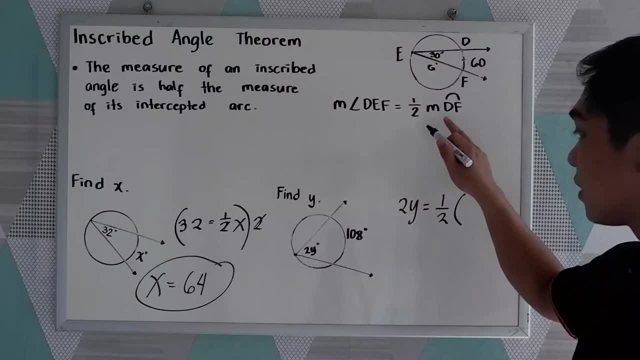 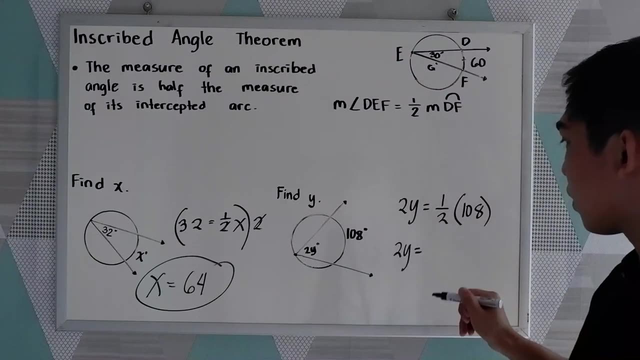 one half of the intercepted arc, which is 108.. So 2Y is equal to 108 divided by 2.. That is 54.. Now to get Y divide by 2. So Y is 27.. Okay. 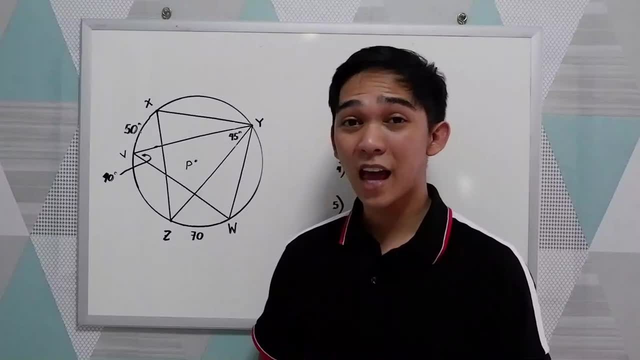 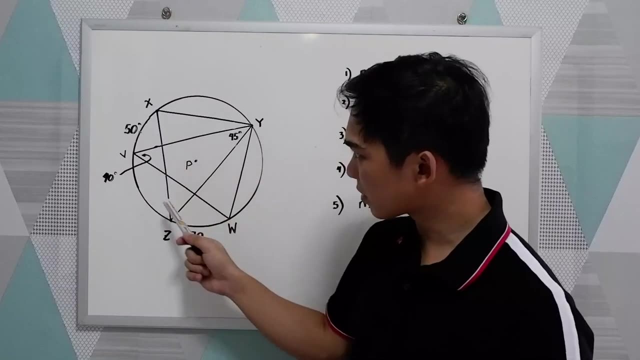 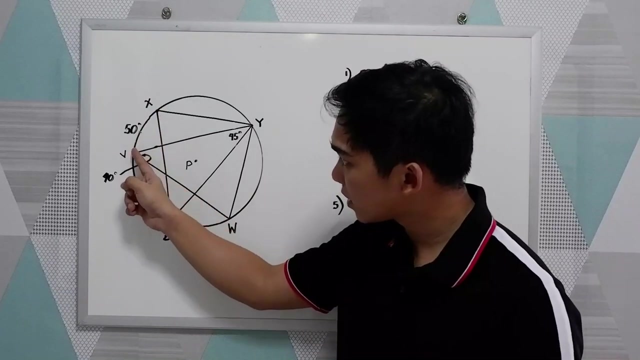 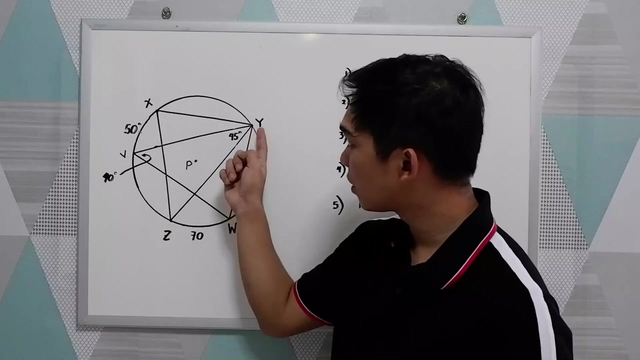 Let us have another example. And now let us have this circle, The circle P, And the following given: We have intercepted arcs and inscribed angles, So we have the given 50 here as the intercepted arc, XV And 40, the measure of angle YVW. 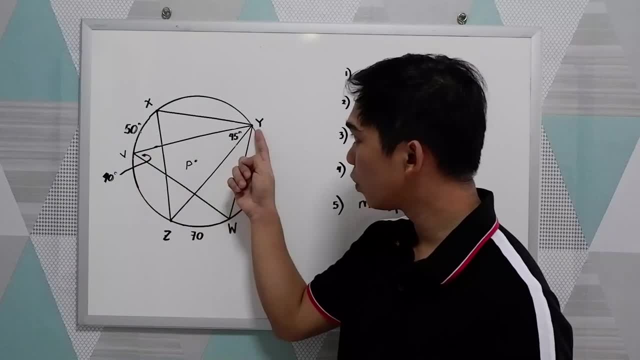 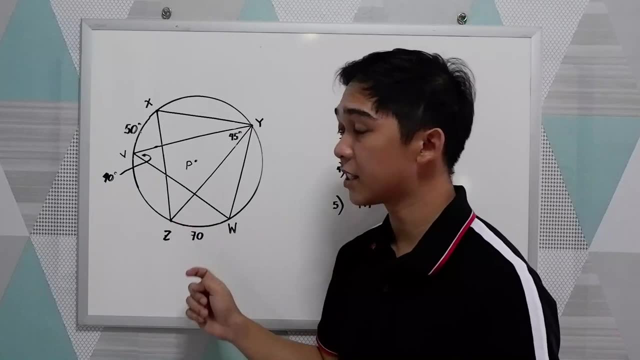 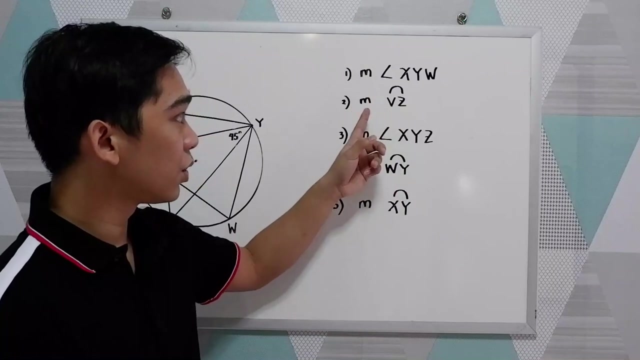 And 45,, the measure of VYZ And intercepted arc, which is 70.. We are going to find the following angles and arcs: Number 1,, 2,, 3,, 4, and 5.. Let us start with number 1.. 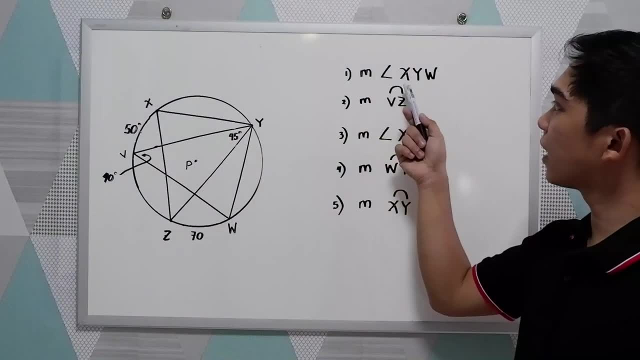 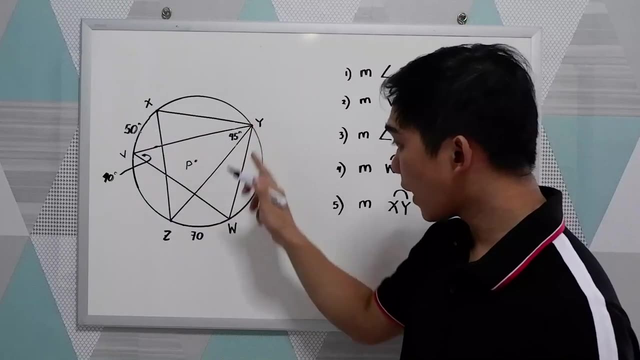 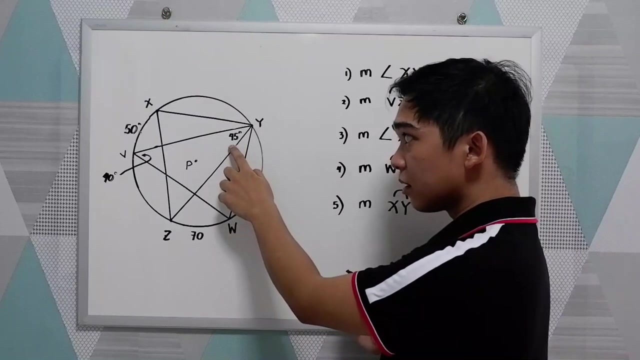 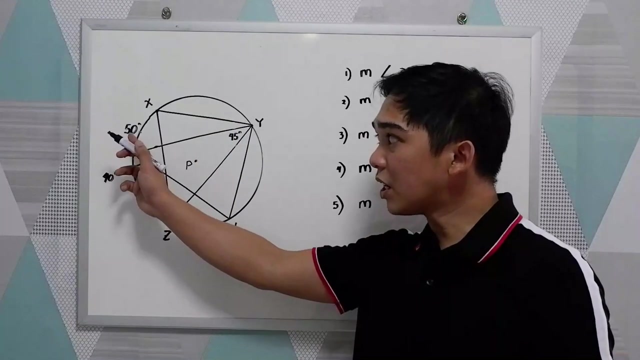 Find measure angle XYW. Where is XYW, XYW, Okay, This angle. So we have 45 here. We are going to find the measure of this angle and this angle. So we have a given here which is 50.. 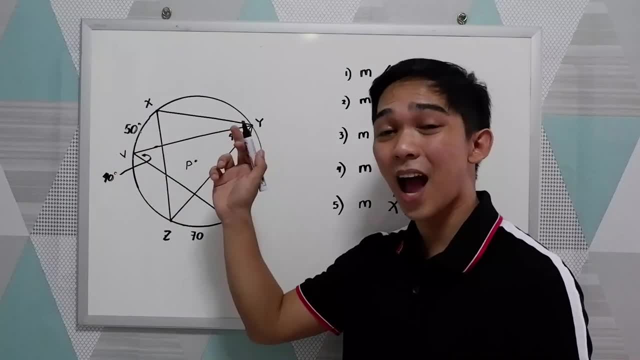 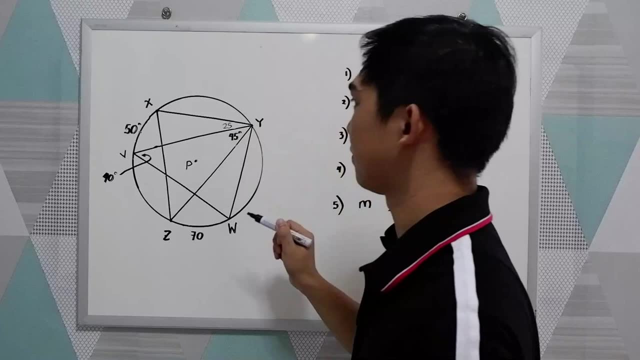 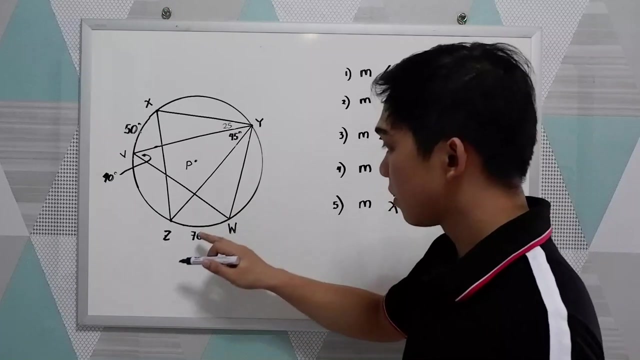 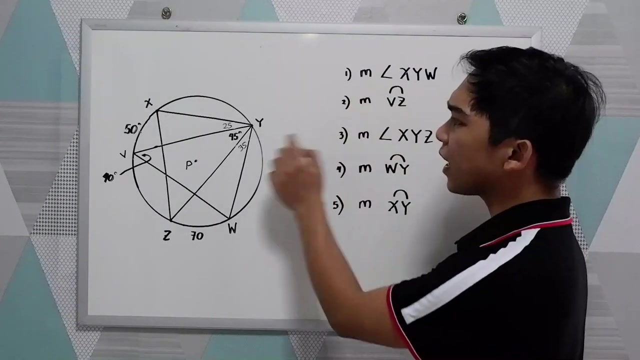 And the measure of this angle is half, Is half of the intercepted arc. So half of 50 is 25.. And this angle is half of the intercepted arc. Half of 70 is 35.. Now to get the measure of the angle, we are just going to add 25 plus 45.. 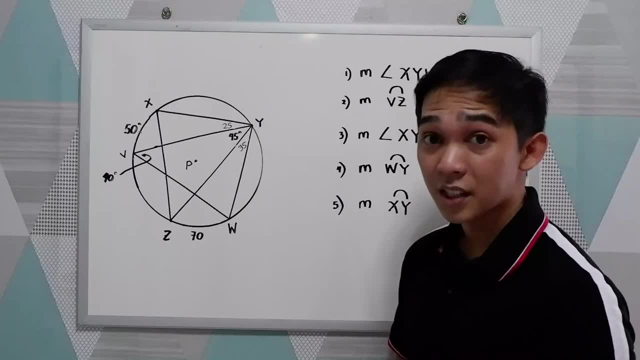 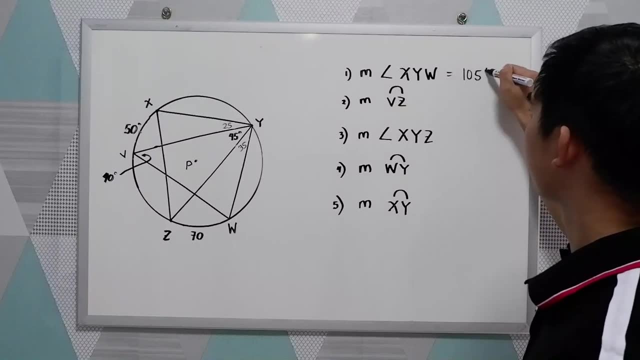 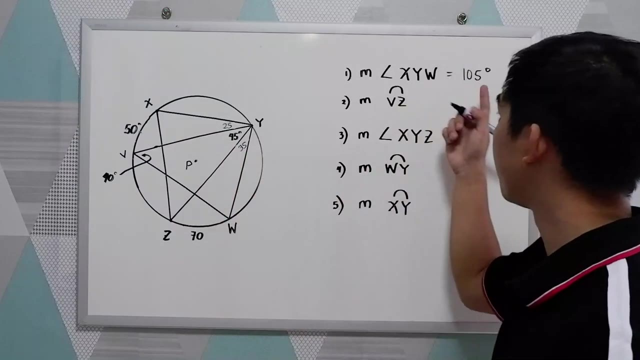 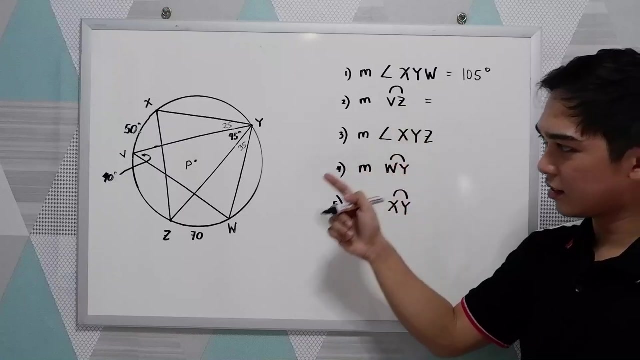 25 plus 45. That is 70.. 70 plus 35. 105 degrees. Again 25 plus 45.. 70 plus 35. 105 degrees. Next, Measure of arc VZ, VZ. Our given is 45, the inscribed angle. 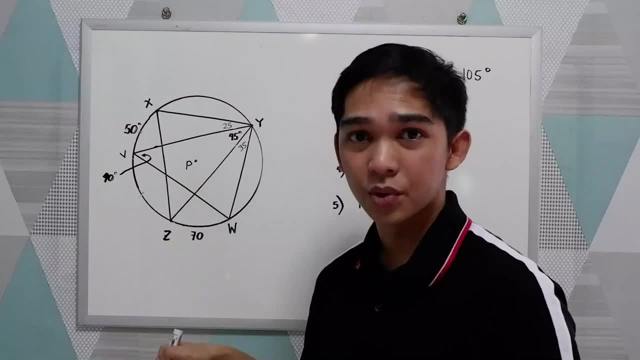 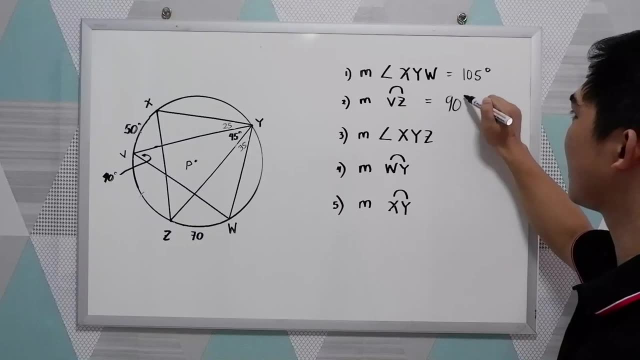 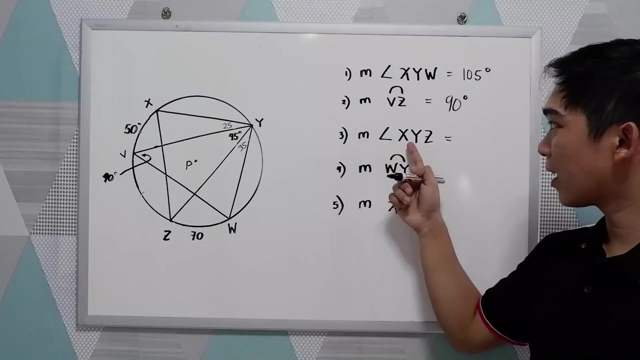 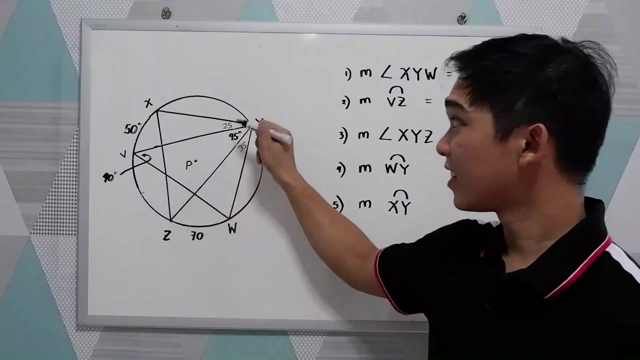 To find the intercepted arc times 2.. So 45 times 2. This is 90.. Okay, 90 degrees. Next, number 3.. Measure angle XYZ. Where is XYZ This angle? So we have 25 plus 45.. 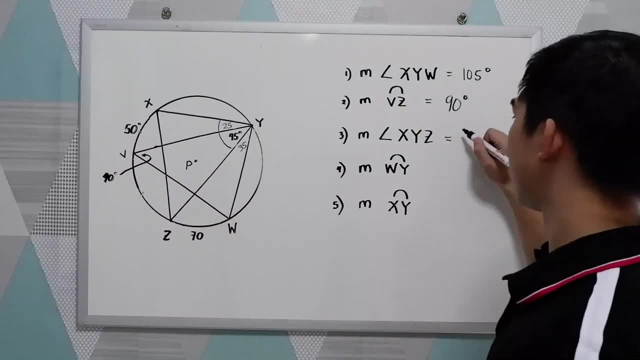 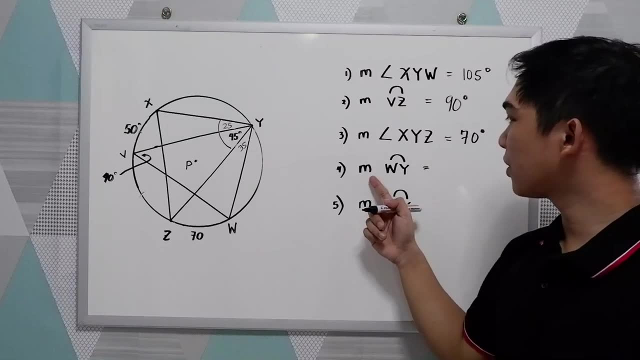 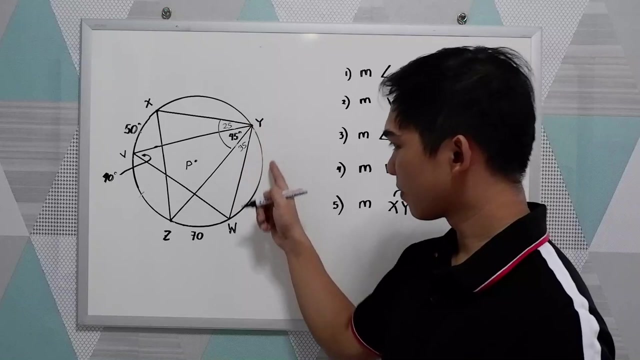 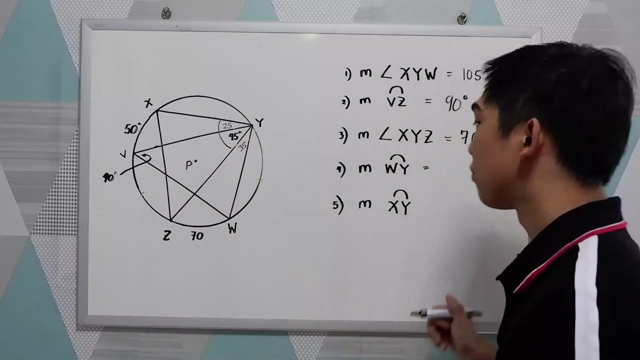 That is, 70 degrees And number 4.. Measure of the arc: WY, WY, WY, We have a given 40.. So times 2.. 40 times 2.. 80 degrees, 90 degrees. 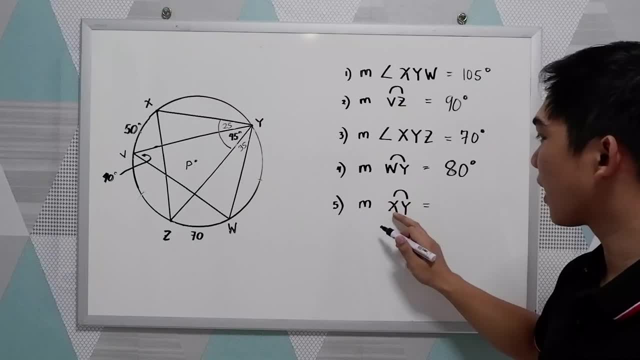 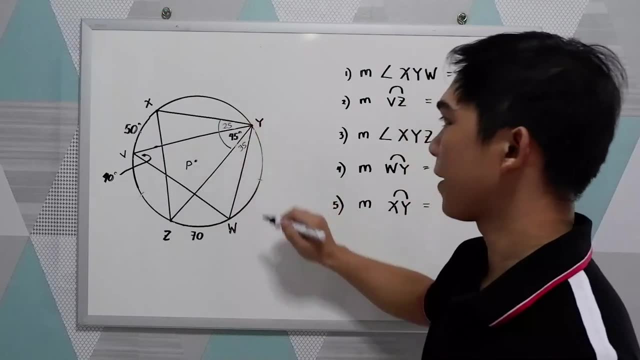 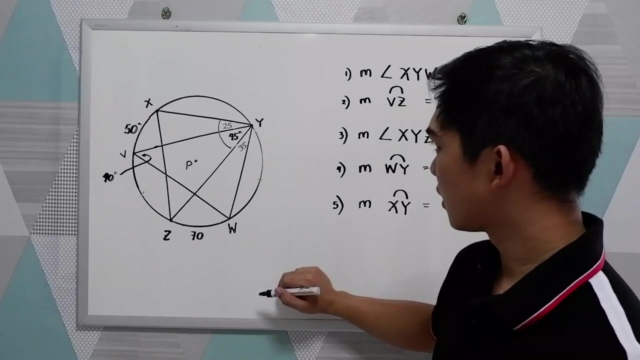 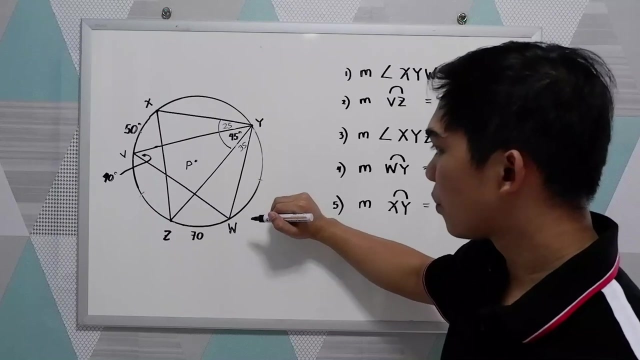 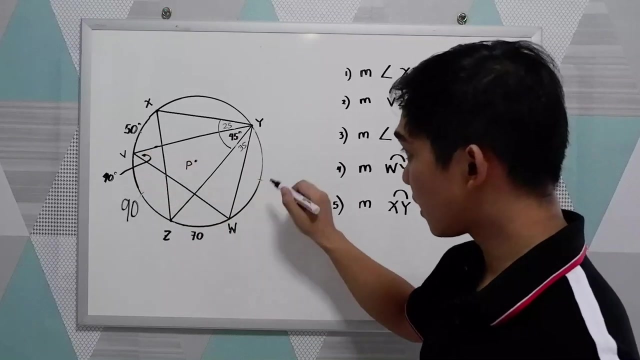 And for our last number, measure, angle Measure, arc XYZ, So XYZ, Okay, So measure of the arc XYZ. So we have 90 here, 80. And this is 80. So 40 times 2.. 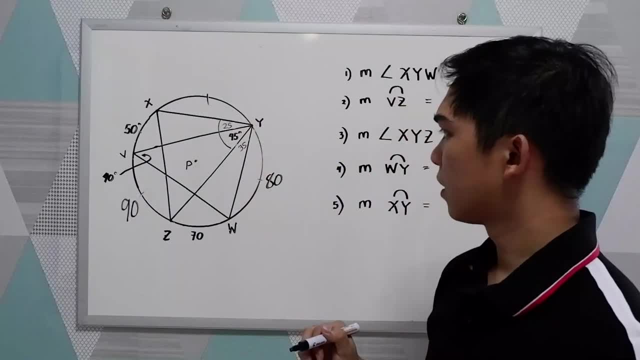 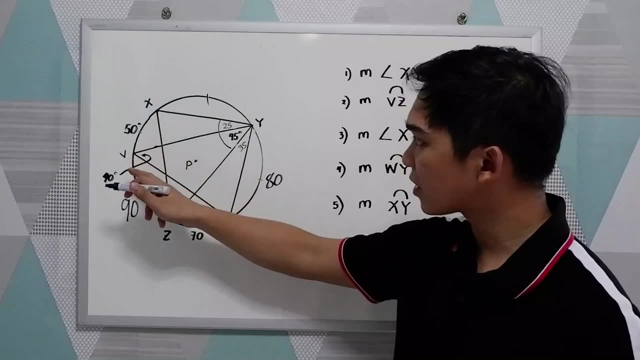 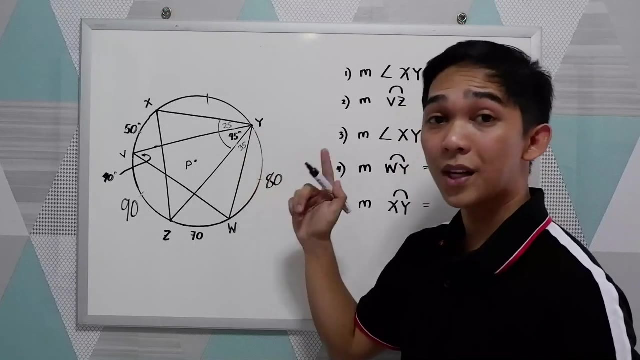 Then this is the missing XYZ. So we study our circle. We have the given intercepted arcs 50,, 90,, 70, and 80.. And to complete our one revolution, we're just going to get the arc XY.